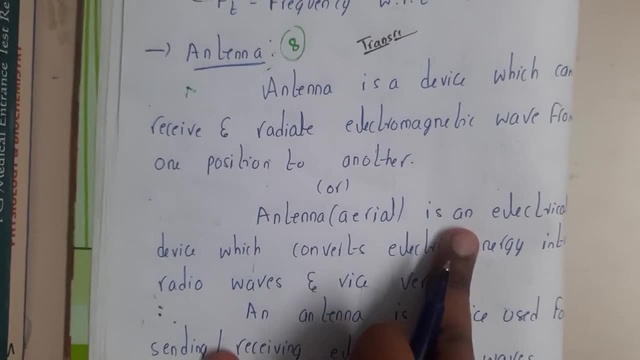 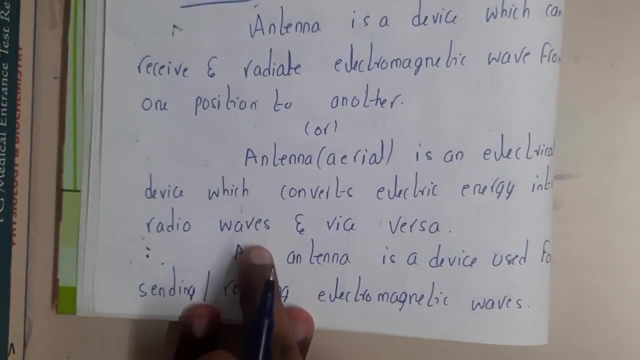 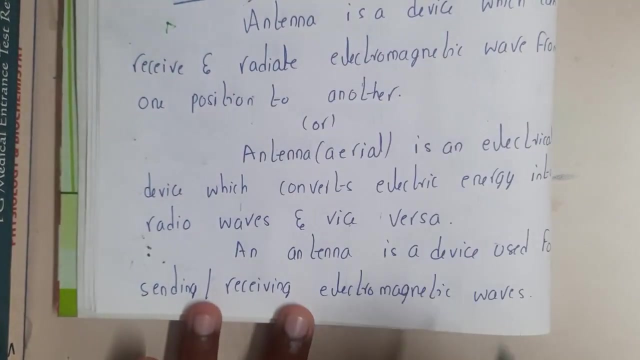 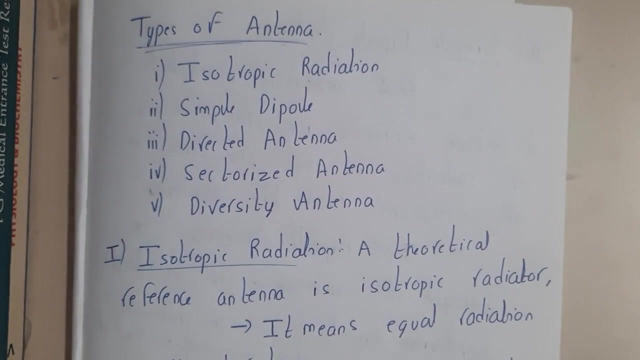 To another. or antennas, Okay, Is an electrical device which converts electrical energy into radio waves and vice versa. So basically, antennas can also be used with radio waves also, guys. Okay, Yes. So an antenna is a device used for sending and receiving of electromagnetic. These are all the definitions. you can say, Okay, Yes. So now let us go through the types of antennas. So, basically, antennas work in different, different ways, guys. So, if you want, I'll be just giving you an overview of each and every one, Then I'll be explaining you. 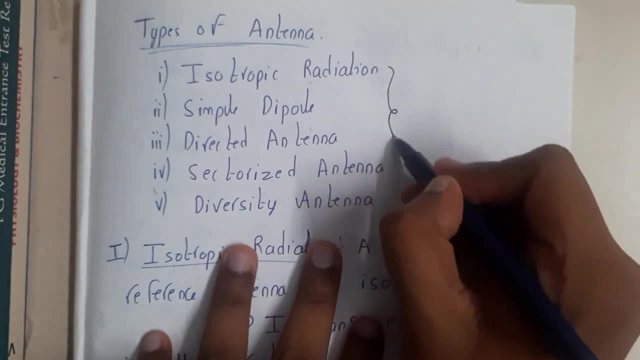 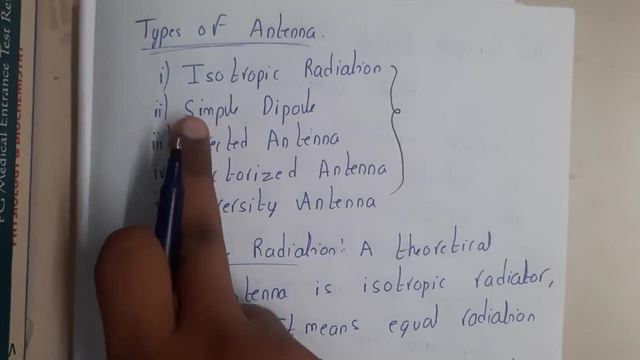 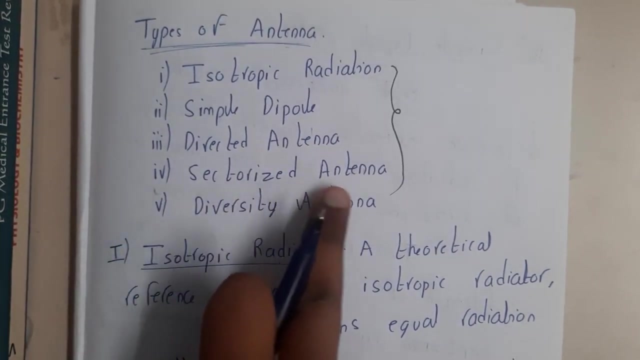 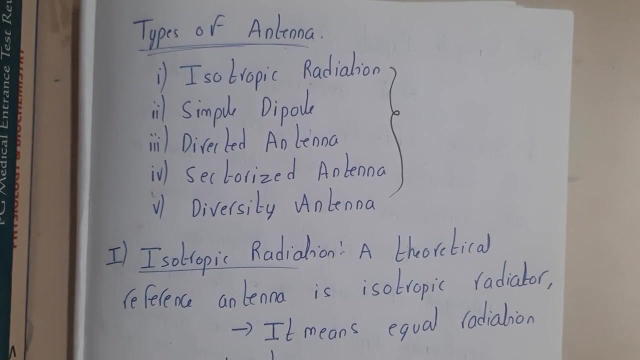 in detail, guys. Okay, Yes. So these are all the five different types of antennas, you can say. So the first type is nothing but isotropic antenna, Okay. The second type is a simple dipole antenna. The third type is a direct directed antenna. The fourth type is a sectorized antenna. The fifth type is a diversion antenna- Okay. So in this lecture let us go through the first three types. After that, in the next lecture, we'll be going through the last two types, guys, Okay, Yes, So I'll be just introducing the first. 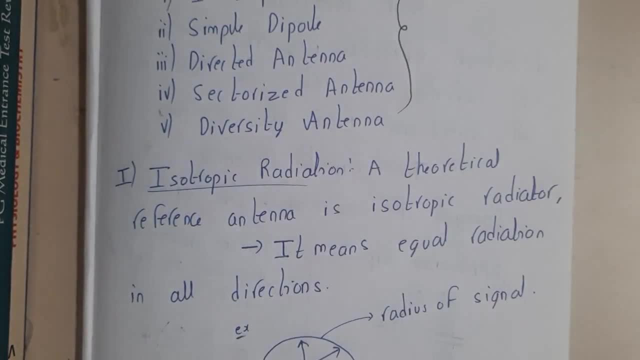 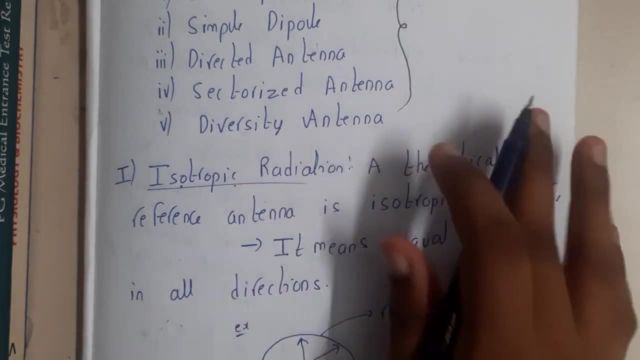 one I'll be explaining in my own words. Then I'll be going through the concept, guys, because in that way you'll be remembering it. well, Right, Yes, So isotropic radiator- Right, Yes, So basically, this is some kind of antenna, you can say, which transmits the signal. 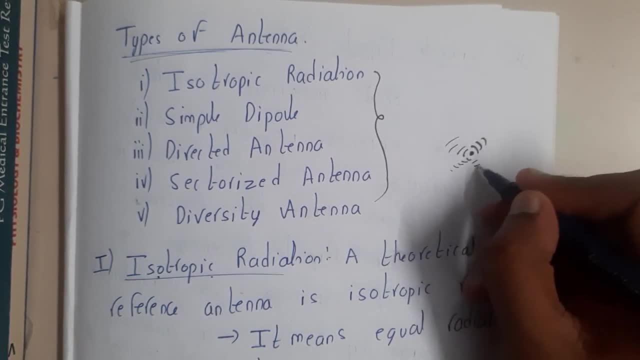 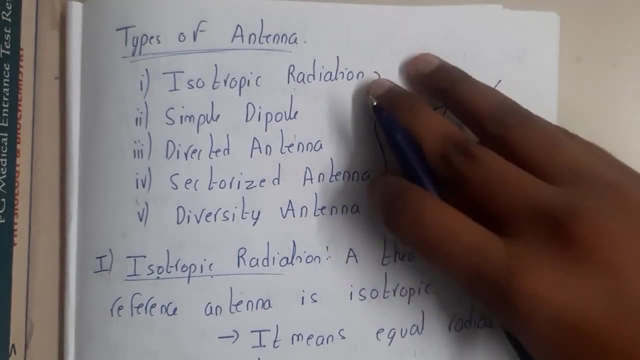 in all the directions, guys. Okay, So there is no fixed direction, like it will transmit only in this direction, or it will transmit only in this direction. So it will transmit in all the directions with the same energy level. So assume that this is the whole region, Right? Yes, So if 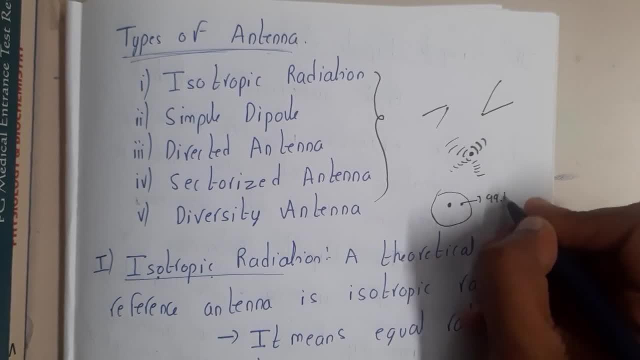 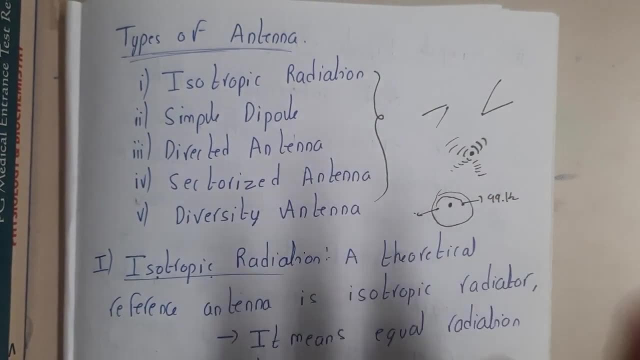 you check here, if the frequency is a 99 hex, So here, exactly at that position from this side also, it will be 99 hex. So in that way it will send in all the directions the same. Okay, Yes, So that is nothing but isotropic radiator guys. So now let us go through the theory. So now you'll be. 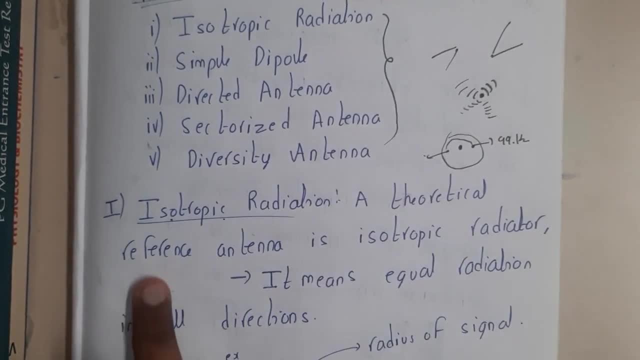 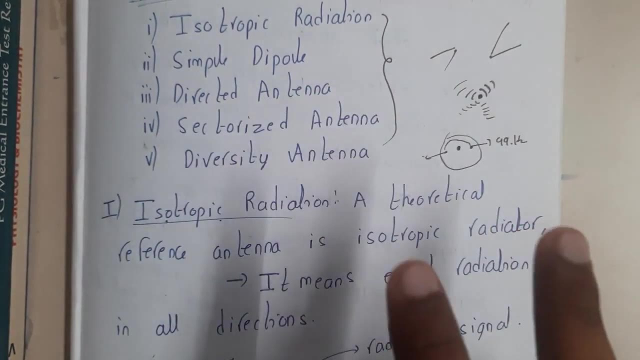 getting a clear idea, guys. So a theoretical reference. So basically, these kind of antennas does not exist, guys. in simple words, you can say: because we are having air around us, Right? Yes, So there could be multiple noises, multiple signals, Right? So that is the reason why there. 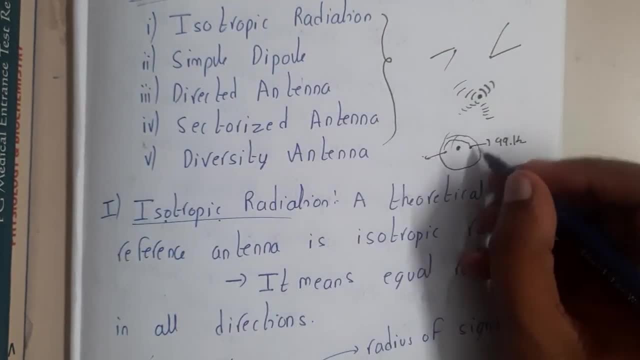 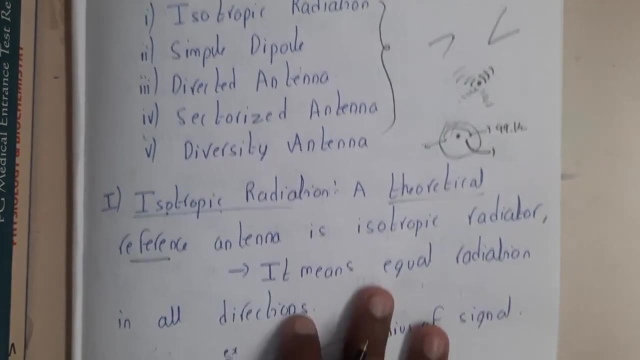 is no chance of sending a signal in all the directions and having it in such a way that it is properly aligned from all places. So that is the reason why this comes under a theoretical reference only. Okay, So it means equal radiation in all the directions. Okay, So here is our 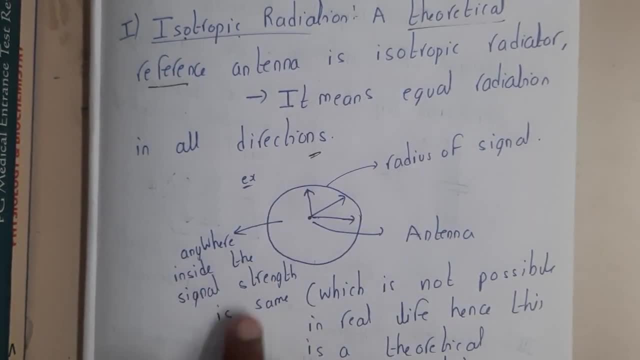 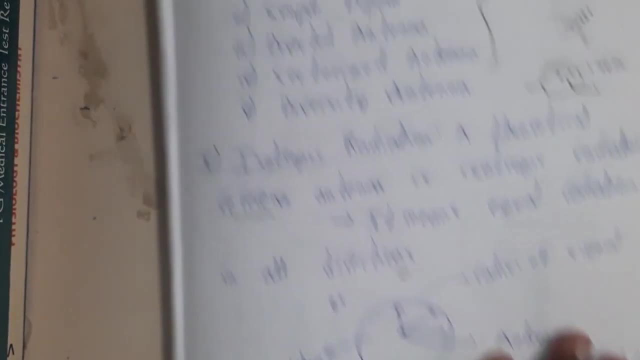 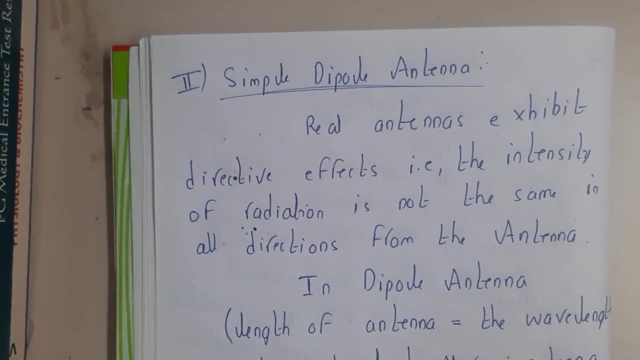 antenna. Assume that this is the radiation, So anywhere inside the signal strength is same, So which is not possible in real life. Hence this is a theoretical reference only, Right? Yes, So let us move to the second type. that is nothing but a simple dipole antenna. So basically, if you ask me, 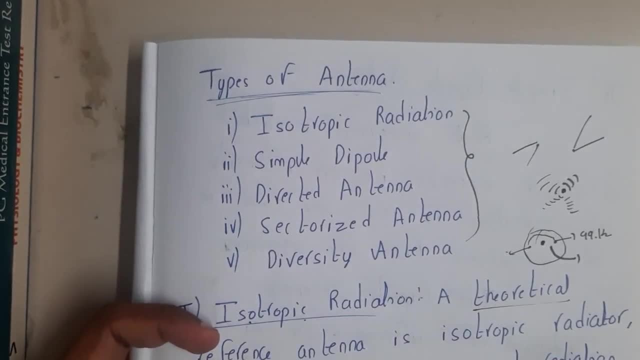 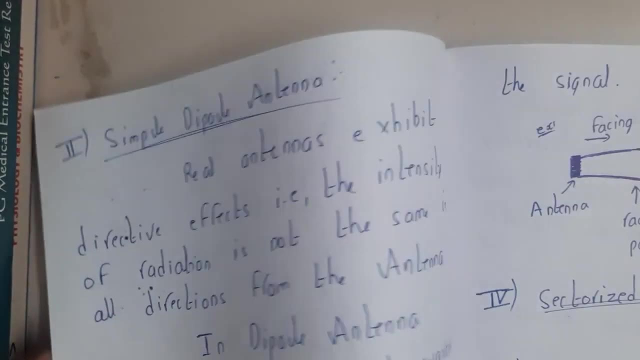 so any of these antennas, you can directly remember them easily, guys, like from the names only. you can say: But this is the only antenna which seems to be a bit complex with the name, Right, Yes, So it is nothing, but the name is a simple dipole antenna, guys. Okay, So it is a real antenna. So I'll be. 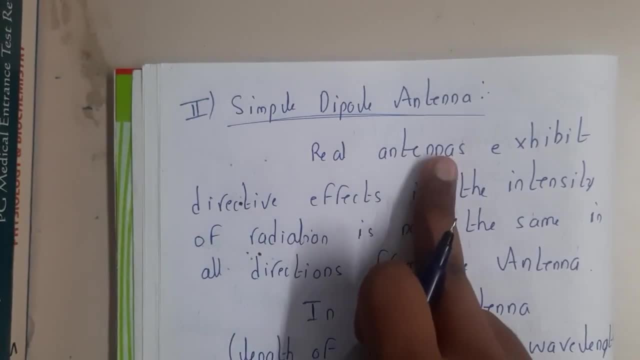 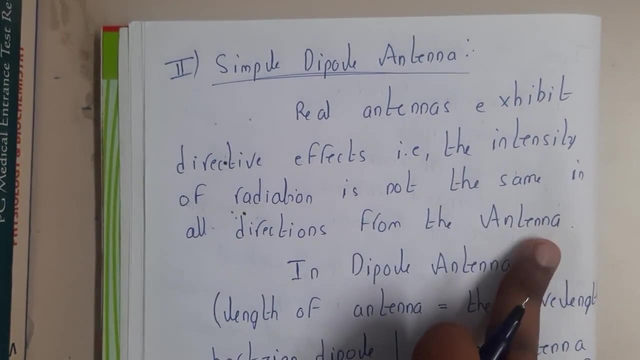 just going through the theory, then I'll be explaining it, guys. Okay, Yes, So it is a real antenna exhibits a directive effect, that is, the intensity of radiation is not the same in all the directions from the antenna. Okay, So basically, previously we discussed about the first type of antenna, Right, Yes, So that is. 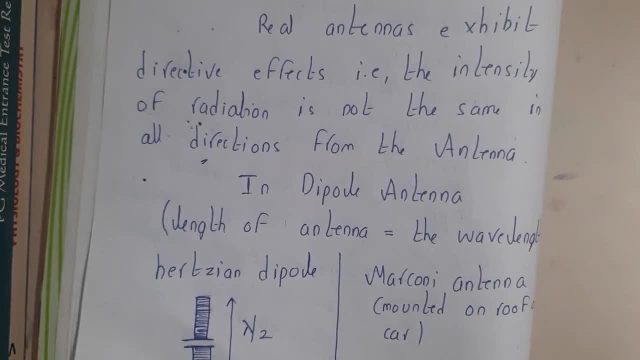 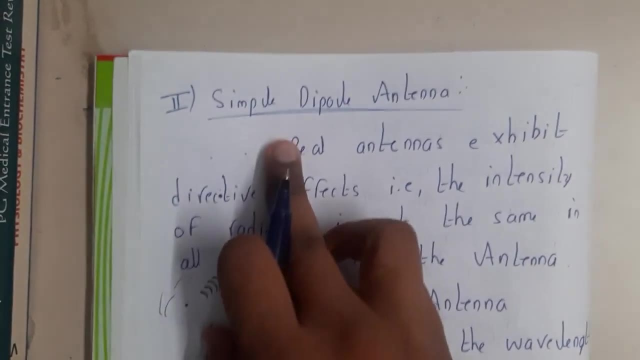 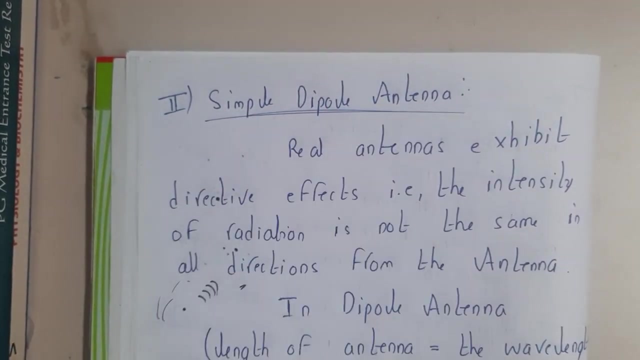 nothing but isotropic radiation or isotropic antenna, you can say So in that the signal strength and everything is the same Right In all the directions. So basically, this is simple. dipole will not do that, guys. So it is just the radiation in one particular direction. So the simple dipole and another best example for it is. so for your CA. 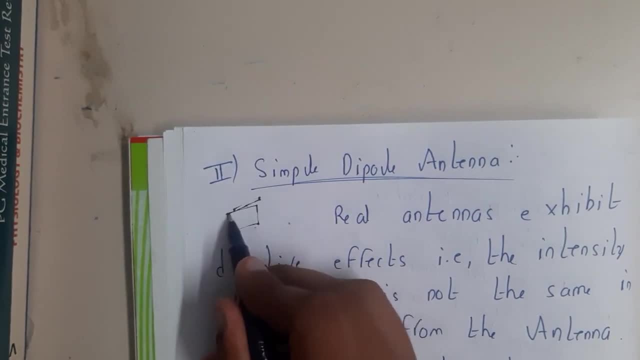 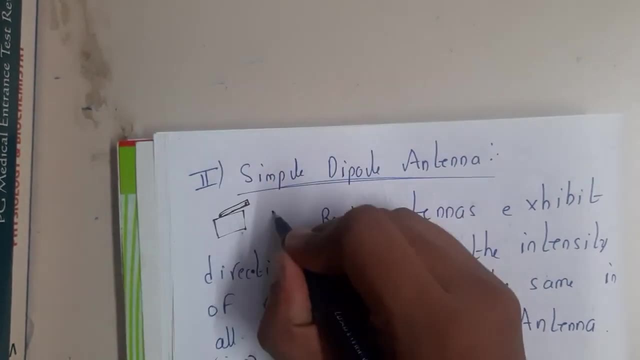 R for our CA. we will be having the signal right. So I don't know what they'll be calling it exactly, but you'll be having a small port right. So whenever you want to turn on that radio, you will be enlarging it So it will really smaller, beworldy. enlarging it so that 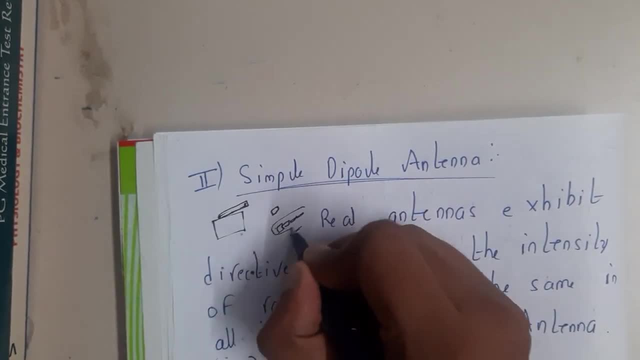 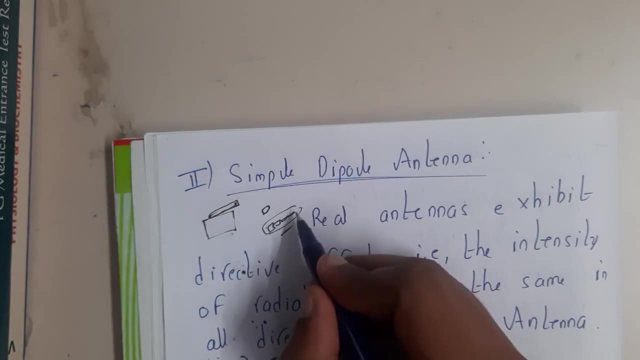 it will be making like this, right, Small, thinner, like this. So this is nothing but what theynu calling. I think you can call it an entity only for now, but if i am wrong, please sorry for that, guys. okay, yes, so basically, this is the example. 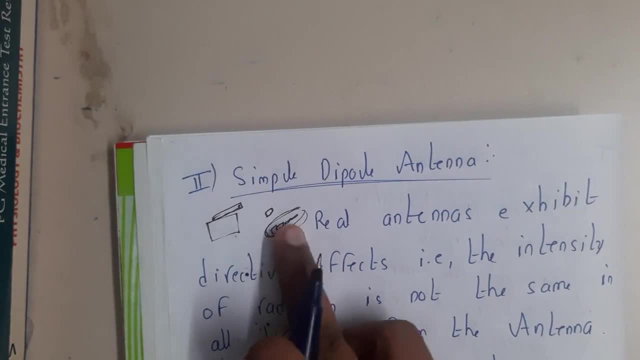 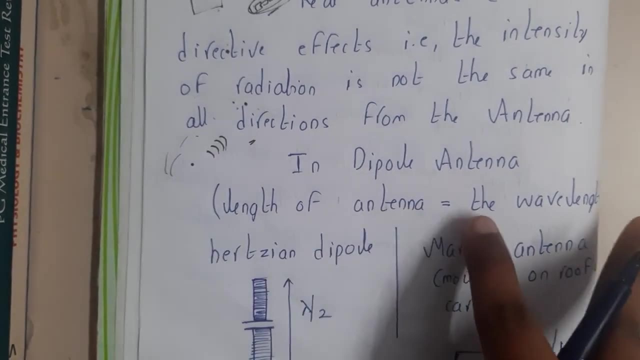 of the simple dipole antenna, guys. okay, so here this length will have a relation, guys. so the length of antenna is equals to the wavelength. so basically, whatever the length of antenna is there, so that up to that much wavelength you can get the day get, or you can connect it to that particular.